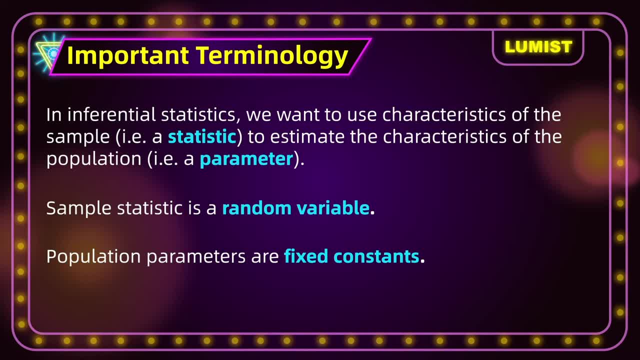 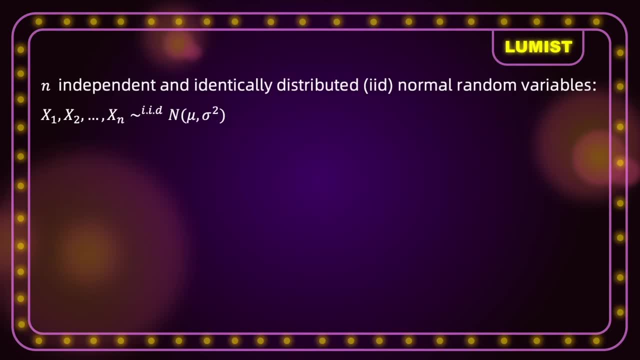 know these of a statistic as a random variable. So let's see the most classic sample statistic here, Sample mean. Suppose our sample are n independent and identically distributed, normal random variables. So that is x1, x2, all the way to xn. follow the normal. 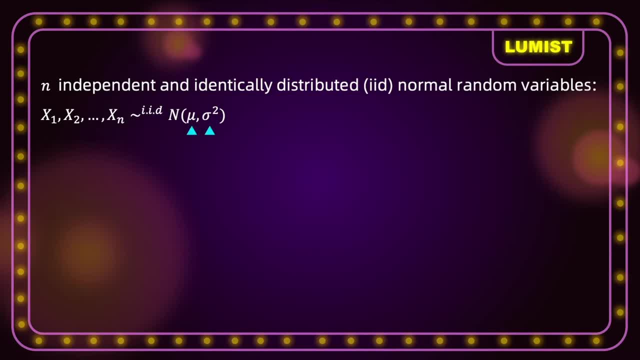 distribution with parameters mu and sigma squared, Then the expectation of xi would be mu and the variance of xi would be sigma squared, even though mu and sigma squared are unknown. So the expectation of xi would be mu and sigma squared, And in other words, each xi might be different, but since they randomly come from the same 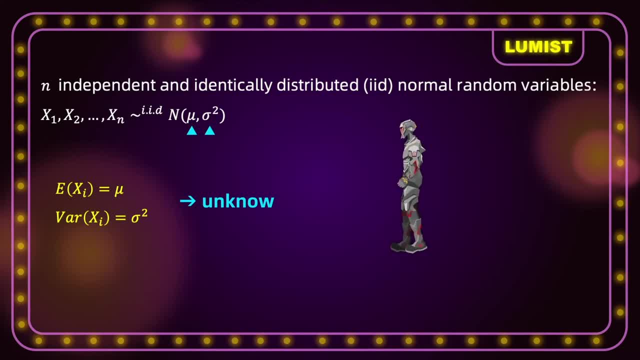 distribution. their expectations are the same. For example, how much would you expect a boy with a height of 1.8m in a certain gym to weigh? Maybe around 180lbs. Then how about when there's another boy who is also 1.8m in the same gym? How heavy would? 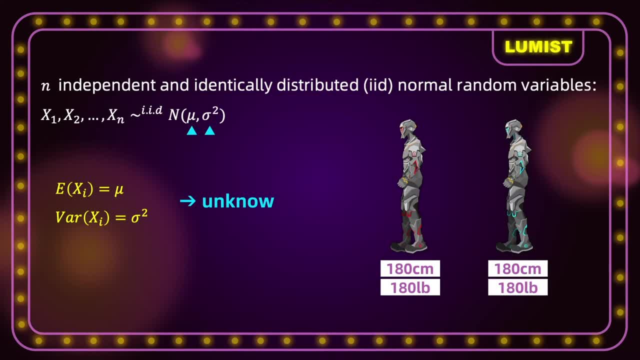 you expect him to be Probably 180lbs too, right The same as the previous boy. Because two boys are from the same distribution, we would expect their weights to be approximately the same. Then let's see what sampling distribution looks like visually. 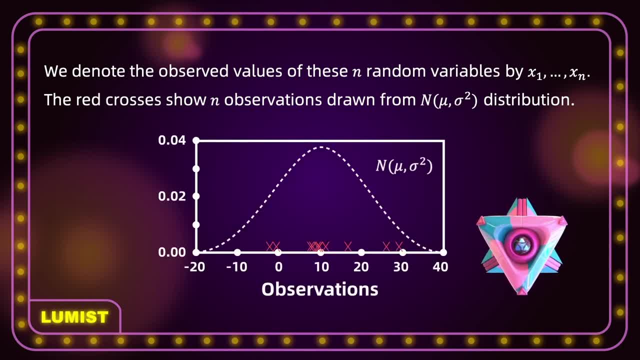 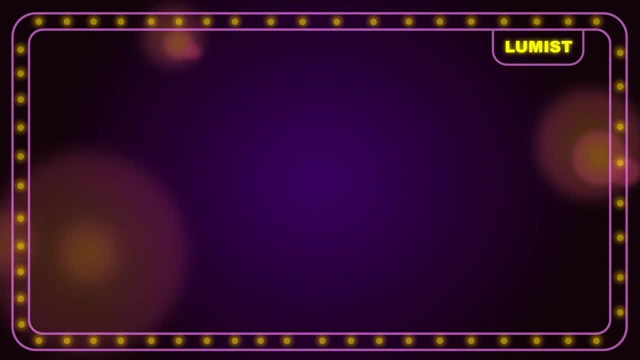 We denote the observed values of these n random variables by x1, x2, all the way to xn. The red crosses here show n observations drawn from a normal mu sigma squared distribution, And again the x-eyes are random variables. The sample mean x bar is equal to x1 plus x2. all the 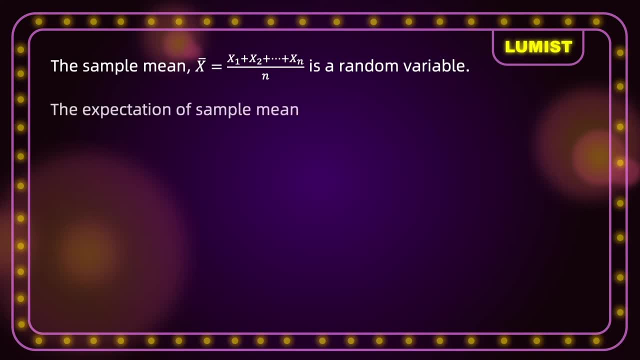 way to xn over n is a random variable. Then we have the expectation of the sample mean, as expectation of x bar is equal to expectation of 1 over n x1 plus 1 over n x2, all the way to 1 over n xn. 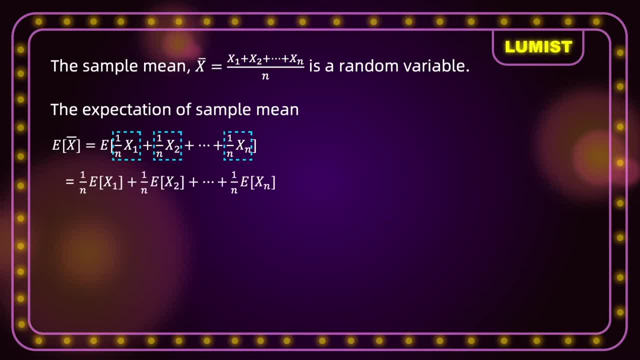 which is just equal to 1 over n times the expectation of x1 plus 1 over n times the expectation of x2, all the way to xn. Remember this property comes from the fact that the expectation of ax plus b is just equal to a times the expectation of x plus b. 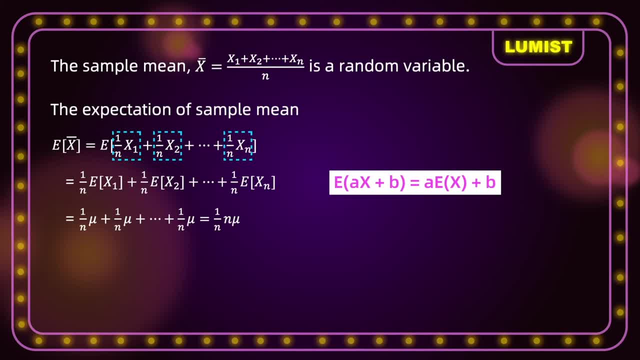 Then we get 1 over n mu plus 1 over n mu, all the way to 1 over n mu n times, because the expectation of xi is equal to mu, The 1 over n and n cancel out, so we're just left with mu. That is, mu is equal to the expectation of x. 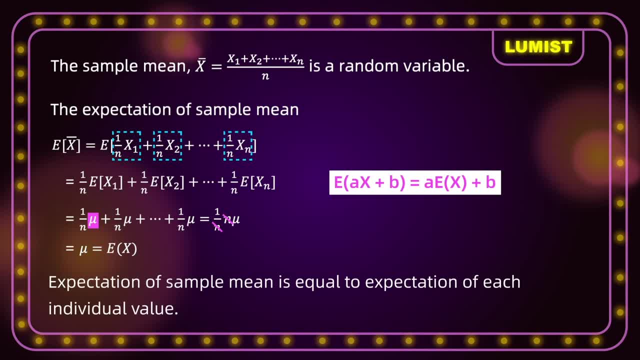 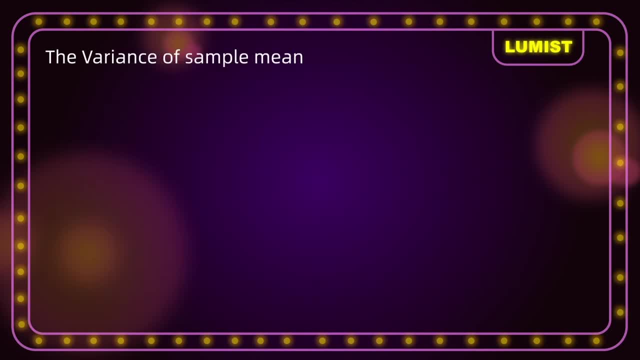 This is a very interesting fact. The expectation of a sample mean is equal to the expectation of each individual value. Now let's find the variance of the sample mean. Remember that variance of x bar is equal to the variance of 1 over n x1, plus 1 over n x2, all the way to 1 over n xn. This is just equal to 1 over. 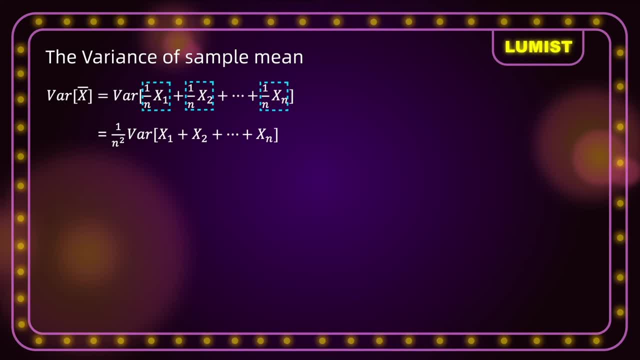 n squared times the variance of x1 plus x2, all the way to xn. because of a very handy property that we learned earlier, which is that the variance of ax is equal to a squared times the variance of x. This here is just going to be equal to 1 over n squared times the variance of x1. 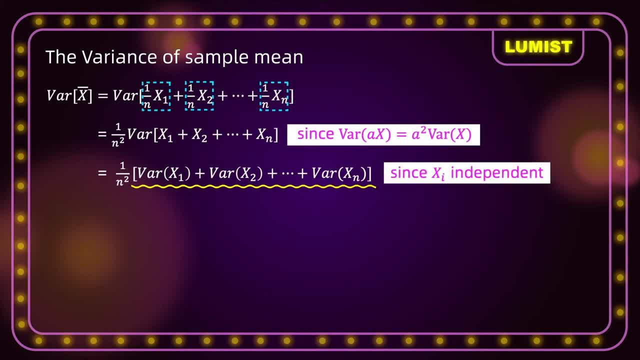 plus variance of x2 all the way to variance of xn. since xi are independent, Then this is equal to 1 over n, squared times n times the variance of xi, and over here n and n cancel out, so we're left with 1 over n times the variance of xi. 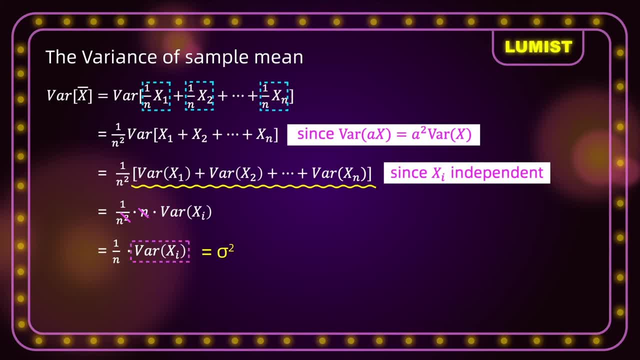 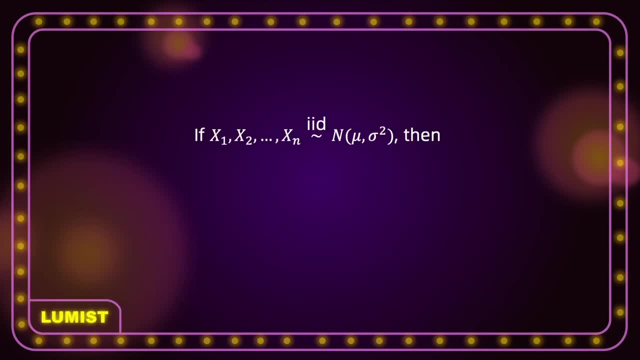 We know that the variance of xi is just equal to sigma squared. so this is just going to be equal to sigma squared over n. So that's the variance of our sample mean. From this we get that if x1, x2, all the way to xn, identically and independently distribute to the normal distribution. 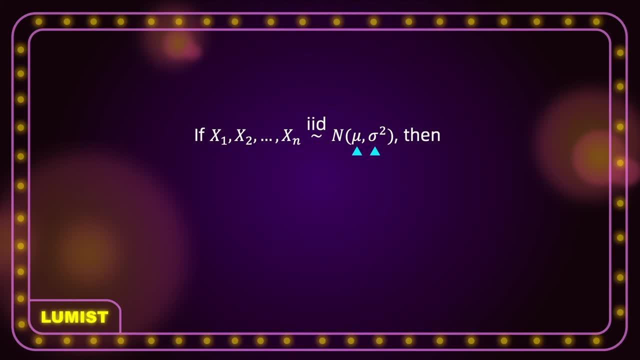 with parameters mu and sigma squared. then, according to the property that the linear combination of normal random variables also follows the normal distribution, we can conclude that x bar follows the normal distribution with parameters mu and sigma squared over n. So here is x bar and here is our variance of x bar that we just calculated. 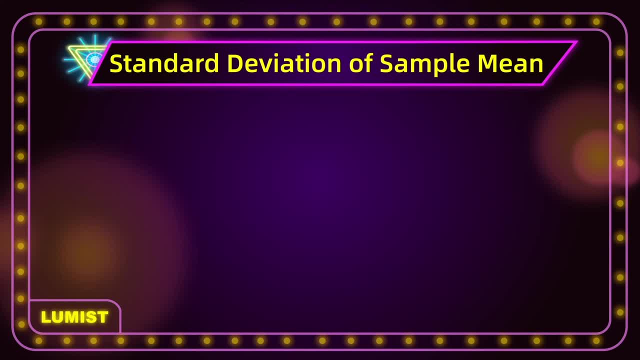 Then, how about the standard deviation of sample mean? Well, it is simply the square root of the variance. Remember, standard deviation is equal to the square root of the variance. Note, however, that here we don't call it standard deviation anymore. Instead, we call it standard error.